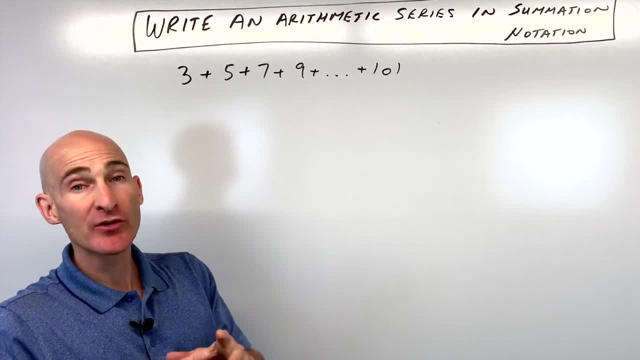 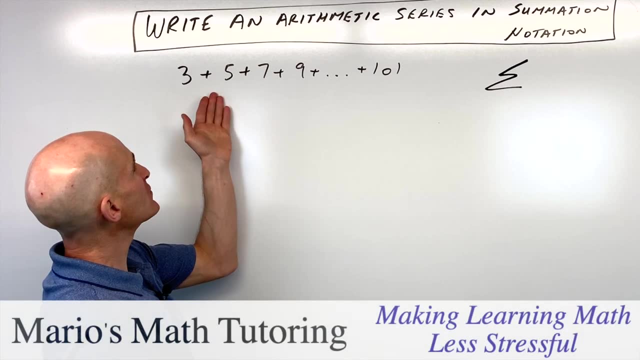 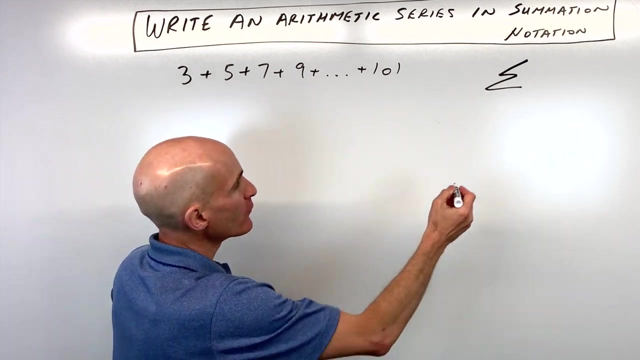 So we're given this arithmetic series- Remember, a series is a sum. We want to write it in the summation notation, That's the sigma notation, And first thing we need to do is we need to find a formula or a rule for finding each of these terms And one of the formulas that you probably learned. 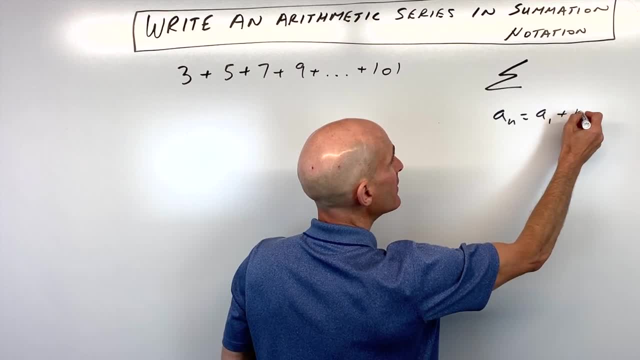 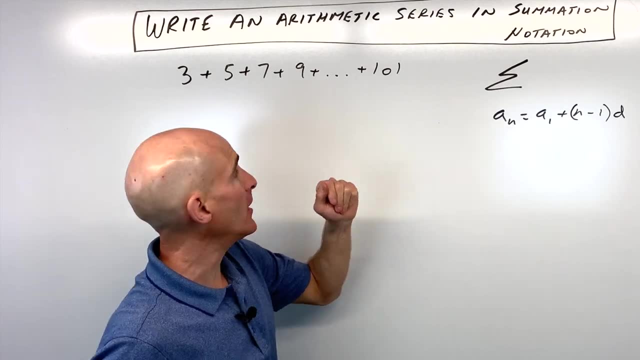 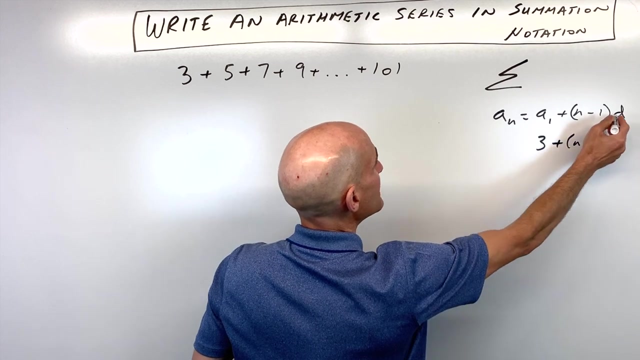 already in your class, is this one here. a sub n equals a sub 1 plus n, minus 1 times d. This is our explicit arithmetic sequence formula, And so what you can see here is that a sub 1, that's our first term- which is 3 plus n, minus 1 times d. That's our common difference. That's what we're. 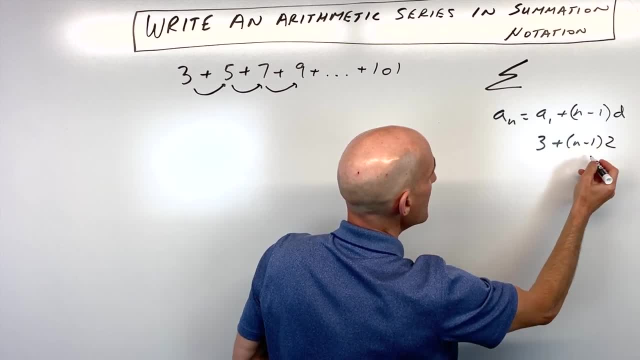 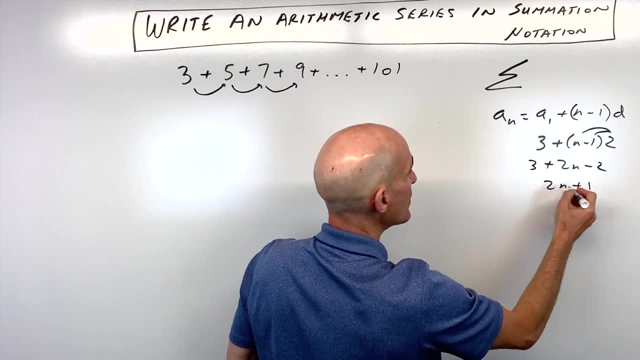 adding to get to the next term, next term. next term, That's going to be 2.. And so if we distribute this 2 in here, we get 2n minus 2 plus 3.. So that comes out to 2n plus 1.. So that's a formula. 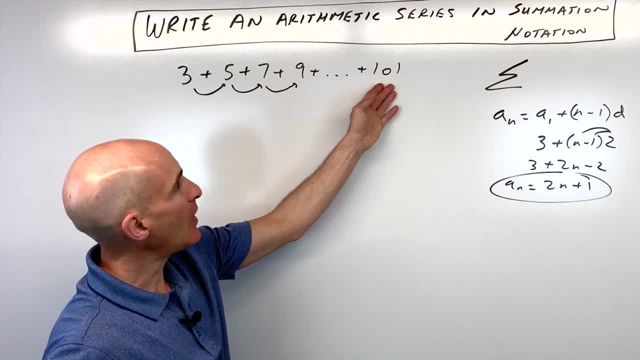 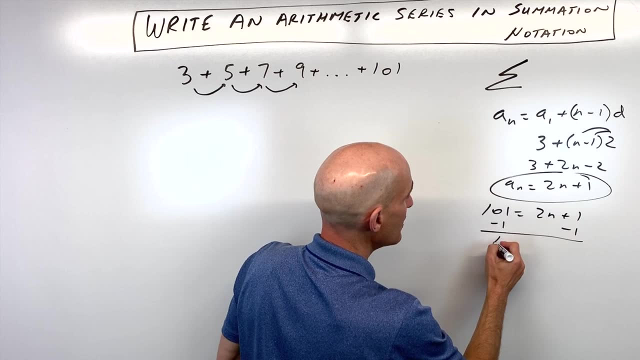 for finding any term. So, for example, if I want to find out, okay, this is a 101.. 101 equals 2n plus 1.. Subtract 1 from both sides: 100 equals 2n Divide by 2.. That means: 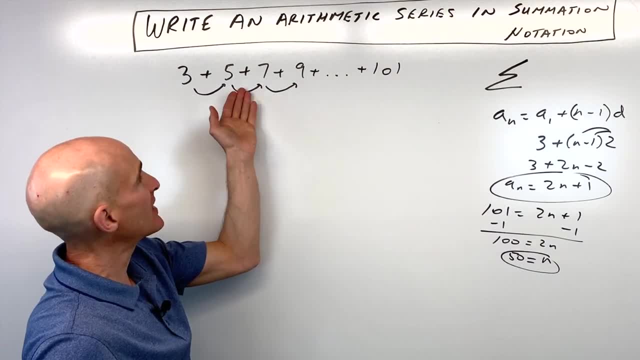 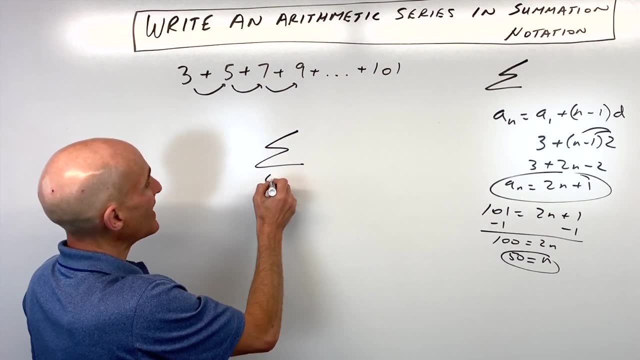 that this is the 50th term, right here. This is the first term, second term, third term, etc. But now how do we write it in the sigma notation, the summation notation? Well, what we're going to do is we're going to say: i equals 1.. Okay, i is our index. It just tells us you know what term. 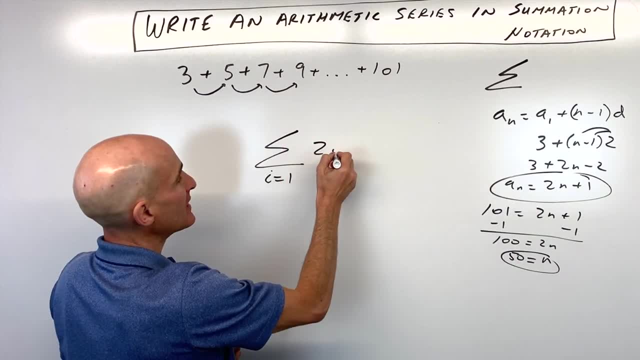 we're working with Here. we're going to put our formula for finding any term. I'm going to make this 2i plus 1.. I'm going to put it in the formula. I'm going to put it in the formula. I'm going to. 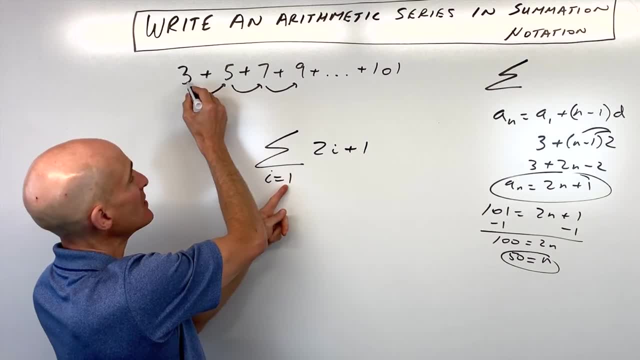 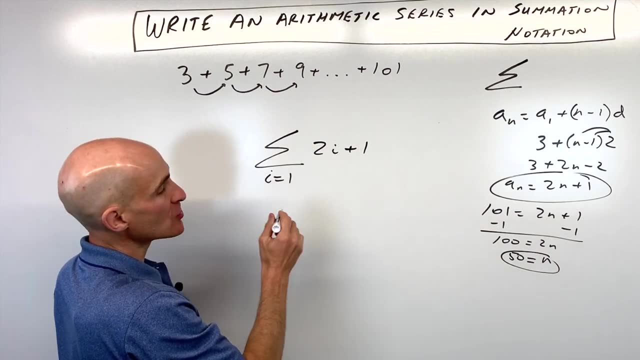 put i plus 1, meaning if I put 1 in for i 2 times 1 is 2 plus 1 is 3.. That's our first term, And then what we do is we work consecutively until we get to this top term, the last term which is going to. 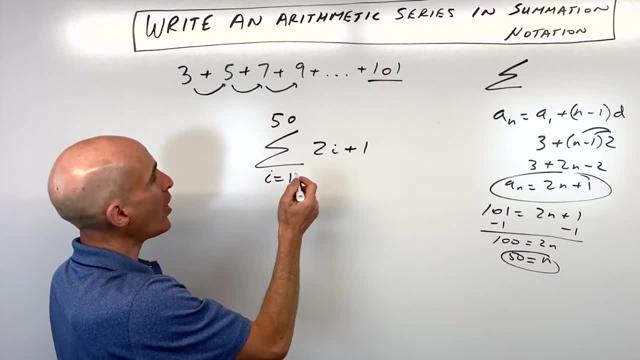 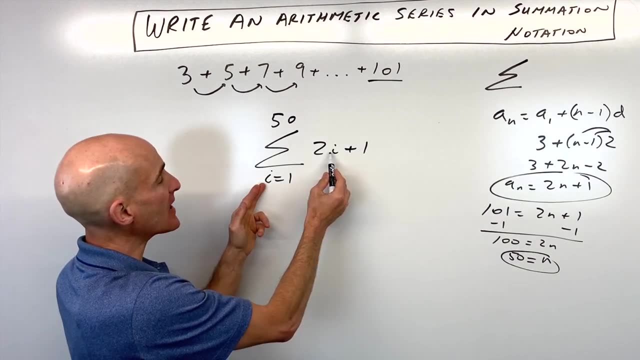 be the 50th term, which we figured out was 101.. So it doesn't matter what letter you use here. You could use i, j, k, n. It doesn't really matter, You just want to make sure that they match. But what? 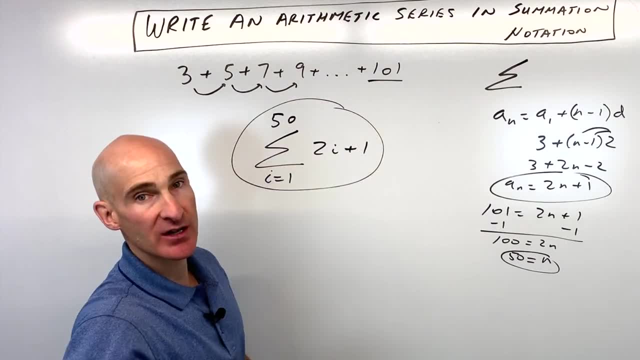 this formula does here for us is it's like a compact way or condensed way of writing out this series instead of writing the equation. So if I put 1 in for i, 2 times 1 is 2 plus 1 is 3.. That's our.